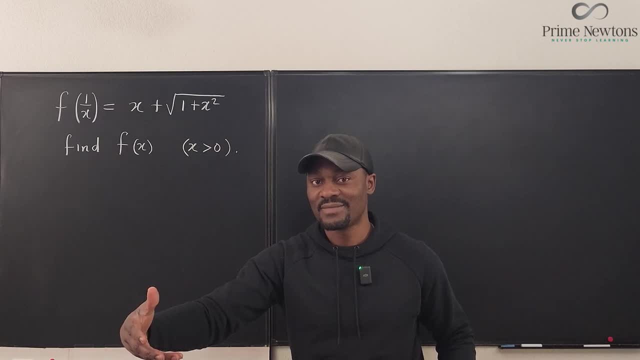 something to F. what does it do with it? Okay, so if you can tell me what F did to this 1 over X to generate this, then you know the answer. But if you cannot tell just by looking, it means you have to do the math. So this is the math I'm going to do And, by the way, 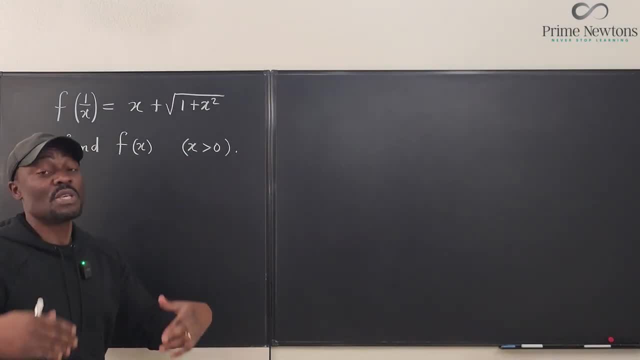 it is for values of X that are greater than 0, because we don't want X to be equal to 0.. Okay, Or maybe because of the square root sign, there might be something that you don't want to do. Okay, So we say that we say let T be equal to this, input 1 over T, or. 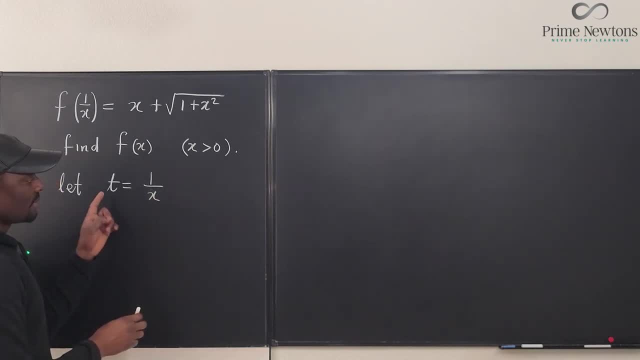 1 over X rather. So we have to get X. Okay, We're going to replace this, but everywhere we see X, we have to replace it with something in terms of T. So that simply means that X will be 1 over T. They're reciprocals of each other, So I'm going to put 1 over T here, 1 over. 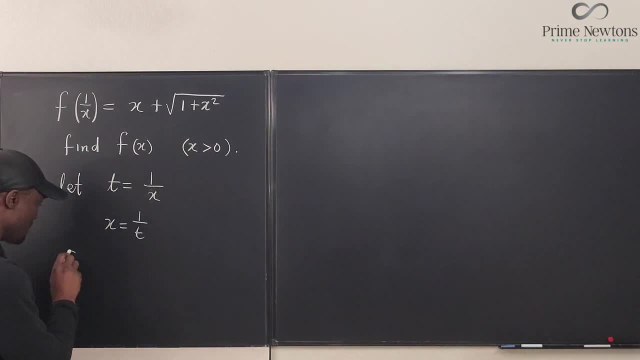 T here and just work things out. So let's start from here. So that means that F of T will be equal to 1 over T Plus the square root of 1 plus 1 over T squared. You can actually leave your answer like this: Okay, But that's not what we want to do. We. 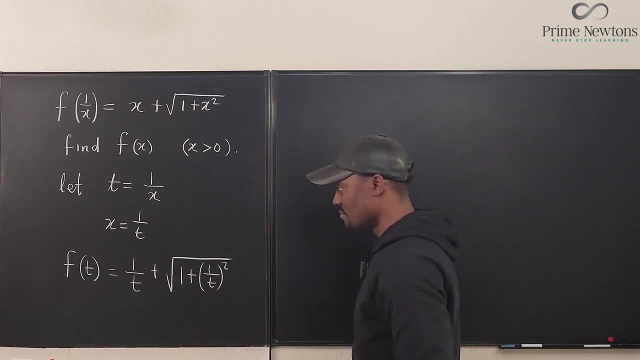 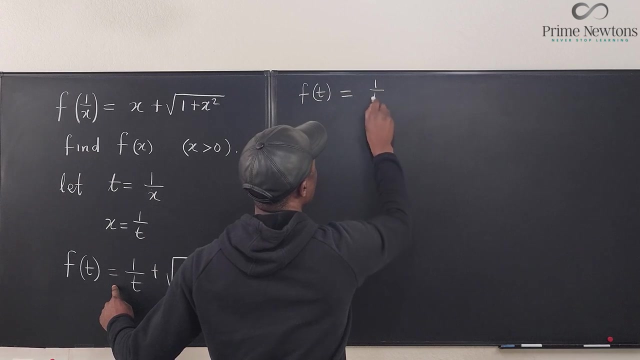 want to actually have something in terms of: yeah, nothing as crazy as this, So let's simplify this. Okay, Now look, 1 over T squared. So we can go ahead and simplify this. Let's say that F of T is equal to 1 over T, plus the square root of 1, plus 1 over T squared. 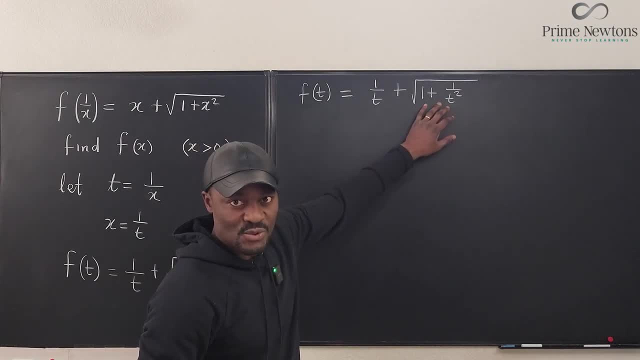 Okay, What's under this parenthesis? we can simplify Because if we make this a common denominator, it's going to become T squared plus 1 over T squared. Okay, Let's write this: It's going to be 1 over T. 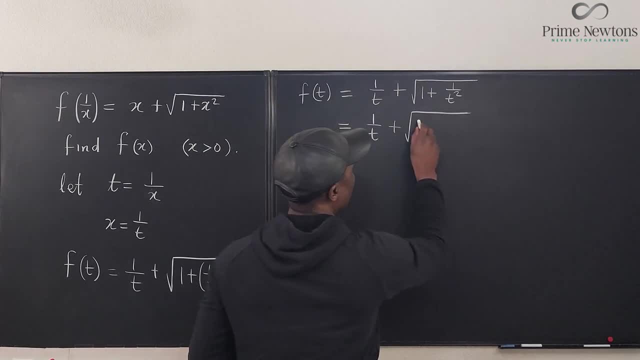 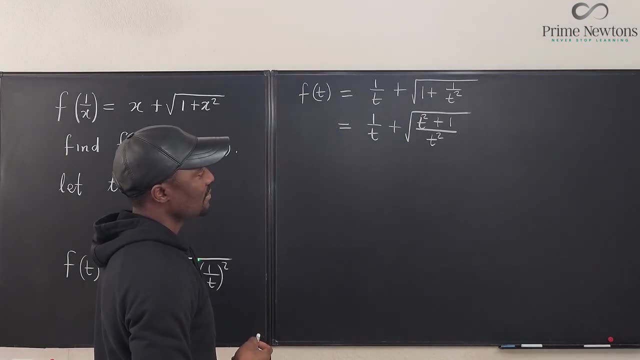 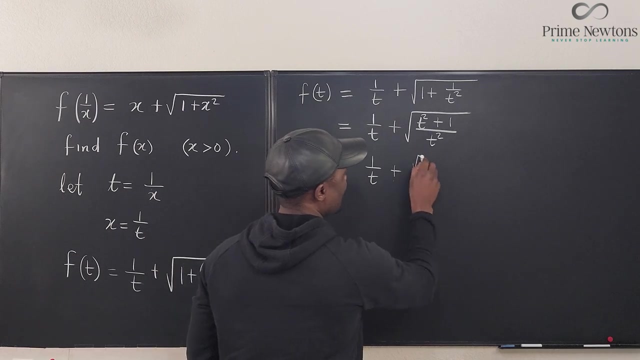 Plug雨 04004 зам más 37ie7合22ص. the square root of t squared plus one over t squared. We can take the square root of the bottom because it's a perfect square. This is going to be one over t plus the square root of t squared, plus one over the square root. 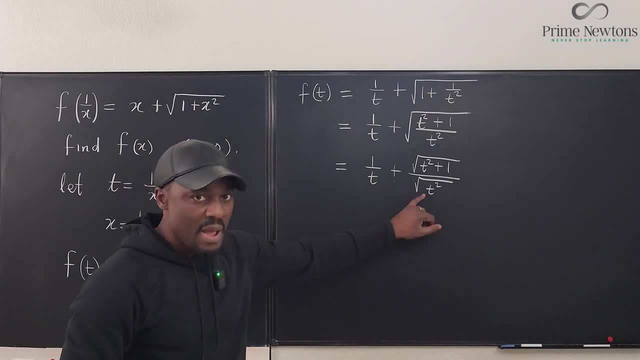 of t squared. Now remember that the square root of t squared is the absolute value of t, so it is plus or minus t, and this is why this information came up. We don't need to worry about plus or minus, because we've been told that any value of x we're dealing with has to be the positive version. Okay, 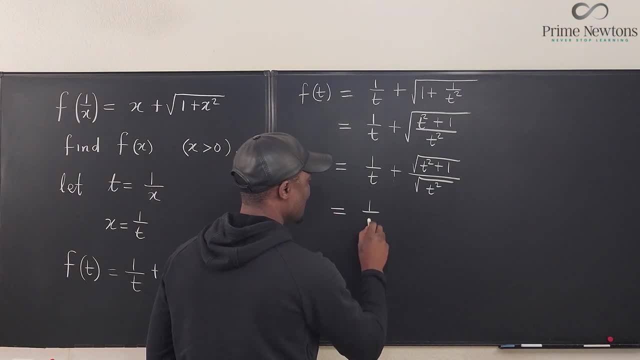 so I'm gonna go here and say this is one over t plus. you see, what we have here is going to be- I'm going to pull this to the side- and it becomes one over the absolute value of t, because that is the square root multiplied by the square root of. let me write one plus t, squared. Okay, well it looks. 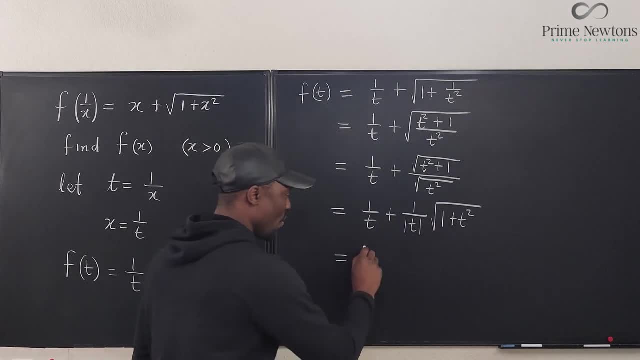 like I am done, because now I can write this as one over t plus one over the absolute value of t. You know, I don't need to repeat that. I think this is my final answer. I just have to say that if I switch this back to x, 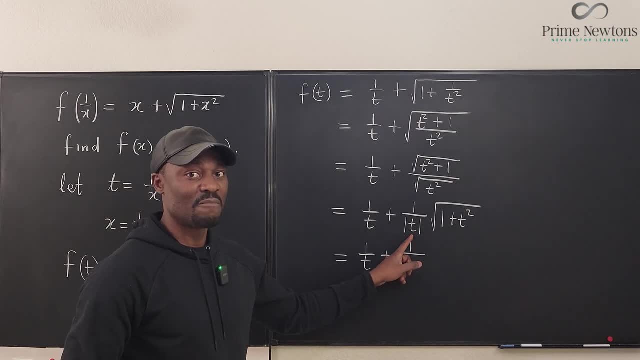 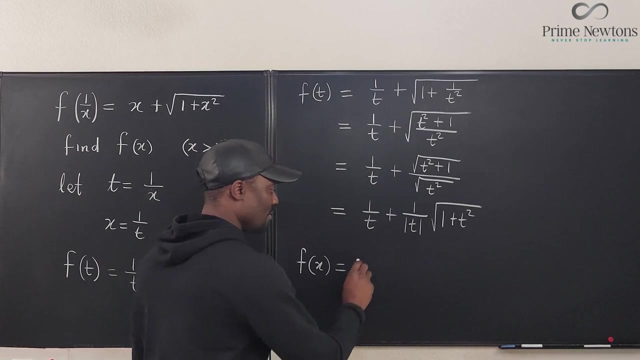 I'm only going to pick the positive version of this because they told us that x is greater than zero. So I'm going to switch this and go to f of x. Okay, that's what I'm going to do. So I'm going to switch back to x at this point and say that f of x is equal to one over x plus one over the. 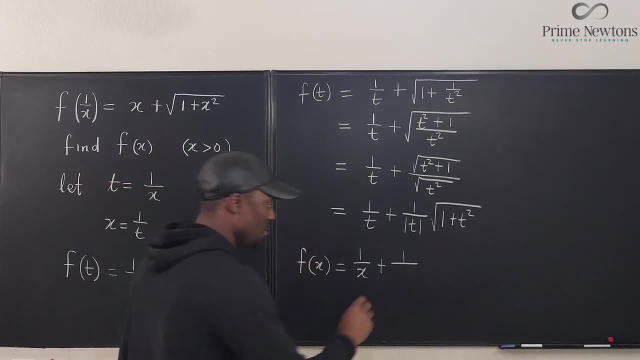 absolute value of x. because x is always a positive number, I can just write one over x times the square root of one plus x squared. So I can factor this out so that f of x is equal to one over x multiplied by one plus the square.